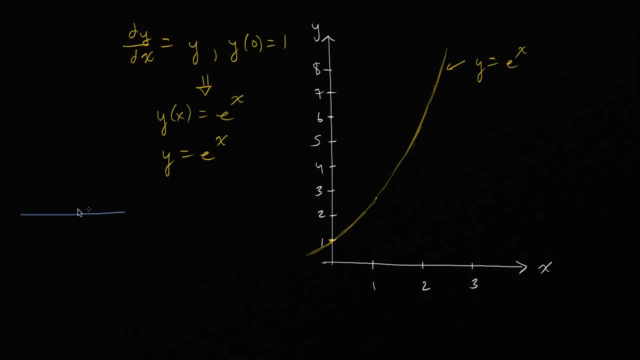 I'm gonna do it over here on the left-hand side. So a little table, So x and then y, with x, y and then dy, dx, And you could set up a table like this to create a slope field. You could just pick all the. 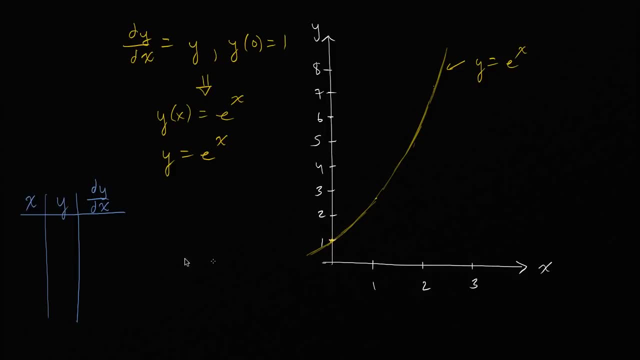 you could sample x's and y's in the xy plane and then figure out for a first-order differential equation like this: what is the slope going to be at that point, and you could construct a slope field And we're gonna do something kind of related. 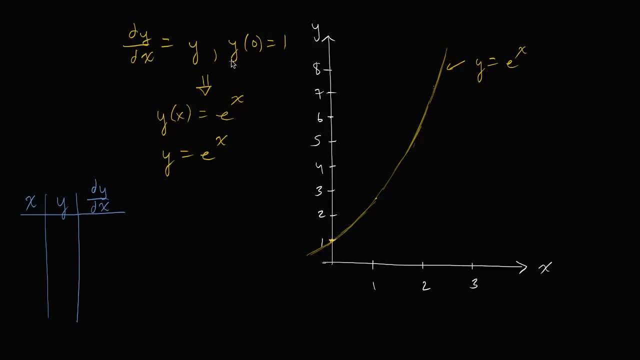 but instead of trying to construct a slope field, we're gonna start with this initial condition. We know that y of zero is equal to one. We know that the particular solution of this differential equation contains this point, So we're gonna start with that point. 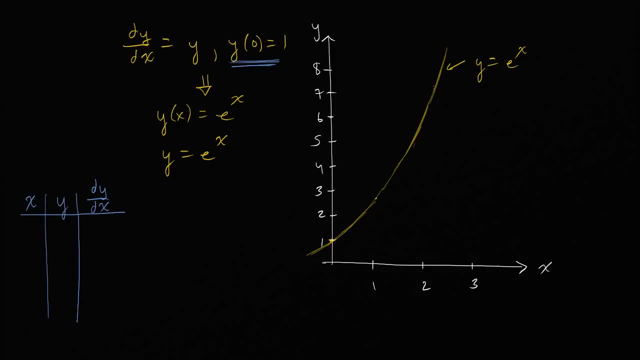 So we're gonna start with: x is equal to zero, and let me do this in a different color. We're gonna start with: x is equal to zero, y is equal to one, which is that point right over there, And we're gonna say: well, okay. 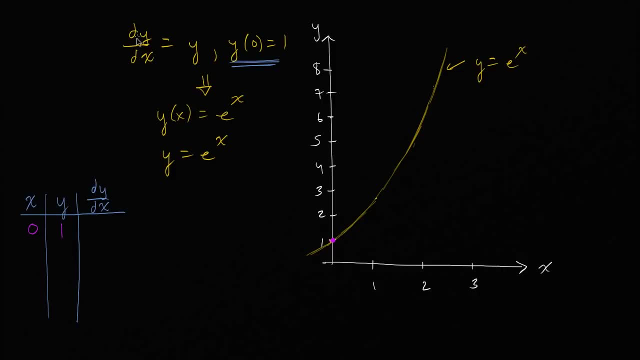 what is the derivative of that point? Well, we know the derivative. at any point or any solution to this differential equation, the derivative is going to be equal to the y value. So in this case, the derivative is going to be equal to y. 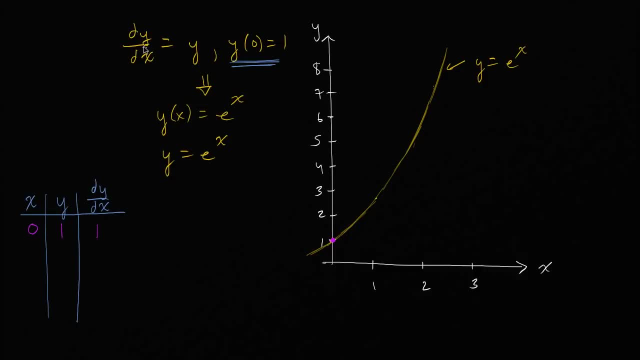 It's going to be equal to one And, in general, if the derivative, just like what we saw in the case of slope fields, as long as the derivative is expressed as a function of x's and y of x's, then you can figure out what the slope. 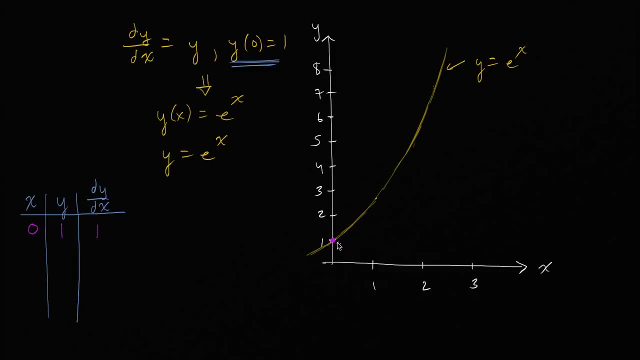 of the tangent line will be at that point, And so you say, okay, there's a slope of one at that point. So I can depict it like that, And instead of just keep doing that at a bunch of points, we'll say, okay, well, let's just 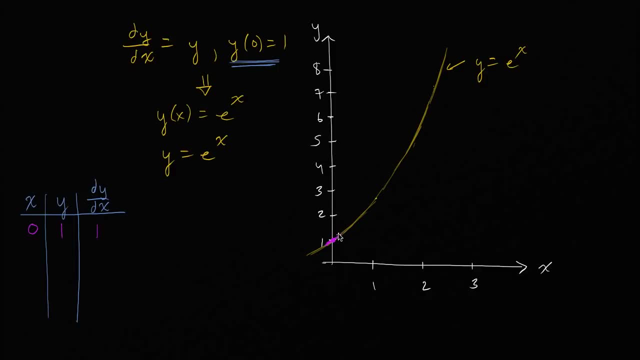 we know that the slope is changing, or it's probably changing for most cases, but let's just assume it's fixed until our next x and then use that assumption to estimate what the next y would be. So what am I talking about here? 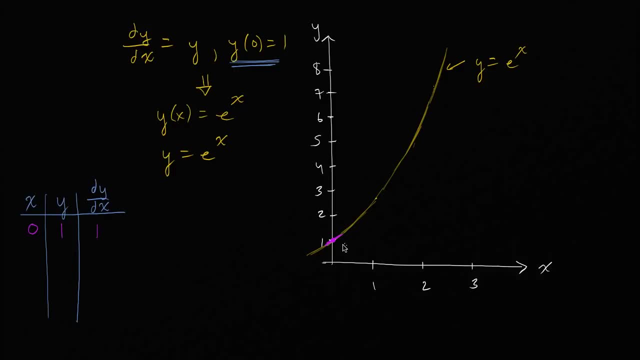 So when I talk about the next x, we're talking about: well, let's just step. let's just say, for the sake of simplicity, we're gonna have a delta x of one, a change in x of one, So we're gonna step from x equals zero. now, 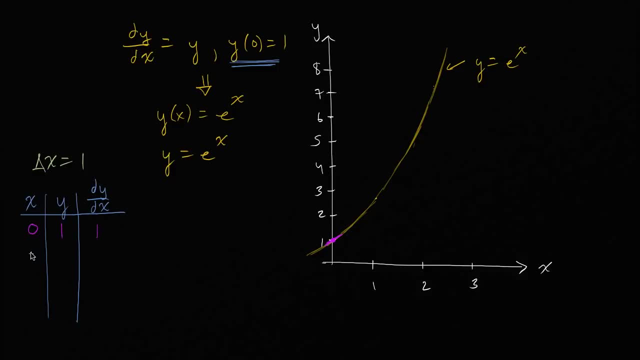 We're gonna now step from that to: x is equal to one. So we're now gonna go to actually let me not use that. I used that yellow color already for the actual graph or for the actual e to the x. So now let's say x is equal to one. 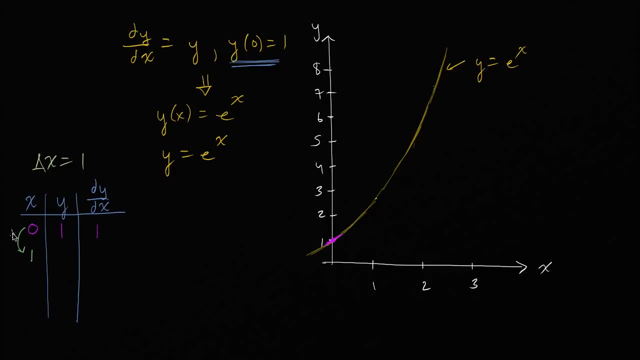 So we've our delta. x is one, So we've just added one here. And what we can do in our little approximation scheme here is, let's just assume that that slope was constant over that interval. So where does that get us to? 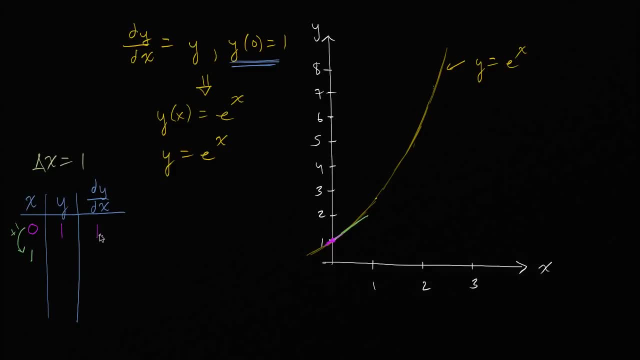 Well, if y was at one and if I have a slope of one for one more for one increase in x, I'm gonna increase by y, by one. So then y is going to increase by one and is going to get to two. 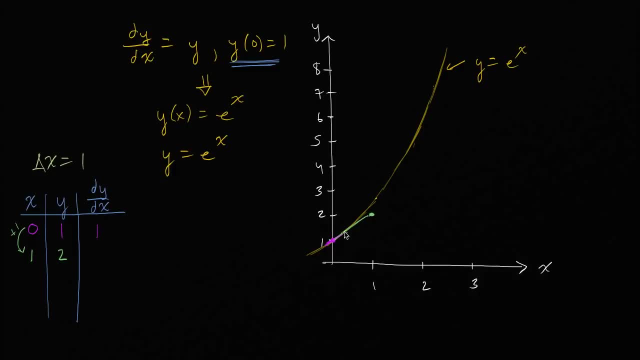 And we see that point right over there, And you already might see where this is going. Now, if this were actually a point on the curve, on the solution, and if it was satisfying this, what would then the derivative be? Well, the derivative is equal to y. 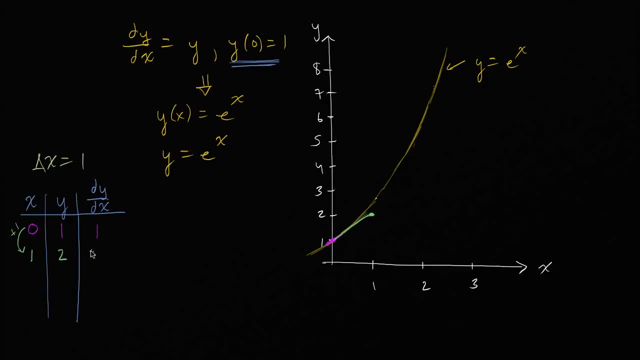 The slope of the tangent line is going to be equal to y. So in this case, the slope of the tangent line is now going to be equal to two, And we could depict that. let me depict that in magenta here. So it is going to be. 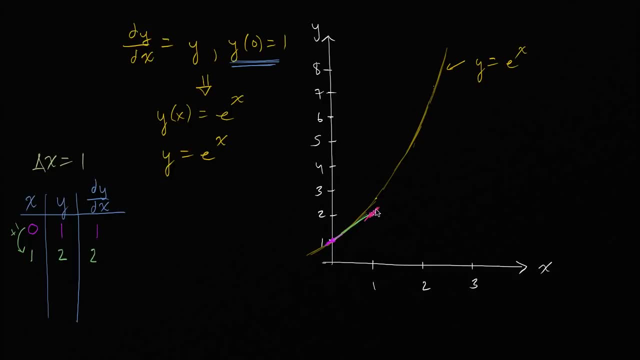 it is going to be two. It's gonna look the slope of the tangent line. there is going to be two. And so what does that tell us? Well, if we step, if we step by our delta x, one more, so now our x is equal to two. 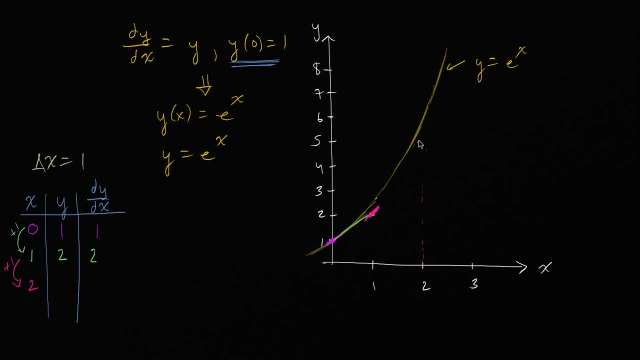 what should the corresponding, what should the corresponding y be? Well, let's see Now: for every one that we increase in the x, in the x direction, we should increase two in the y direction, because the slope is two. So the very next one should be four. 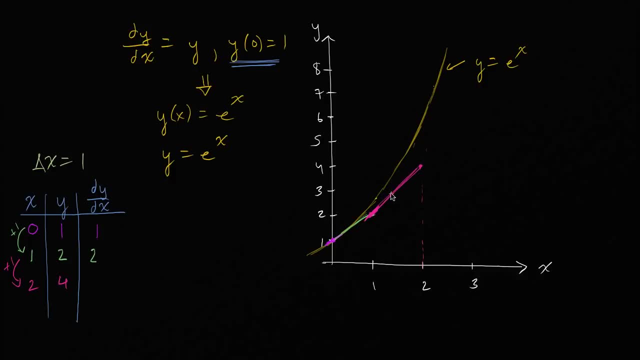 y is equal to four. So we could imagine we have now kind of had a constant slope and we get to that point right over there And now we can do the same thing. Well, if we assume dy dx based on the differential equation, 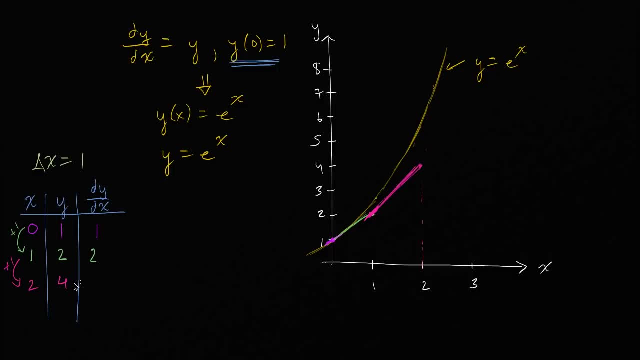 has to be equal to y. we say, okay, the slope of the tangent line there is going to be the same thing as y, It's going to be four. And so if we step our x up by one, if we increment our x by one again, 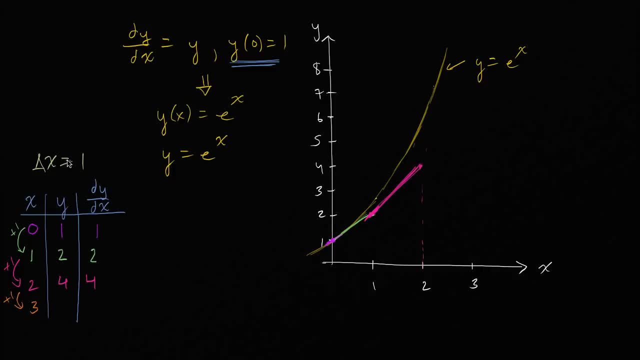 once again, we just decided to increment by one. We could have incremented by 10.. We could have incremented by .01.. And you could guess which one's going to give you a more accurate result. But if we step up by one now, 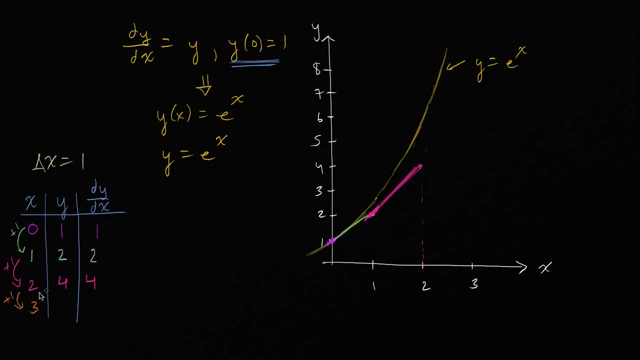 and our slope is four. well, we're going to increase by. if we increased x by one, we're going to increase y by four, So we are going to get. we are going to get to eight, And so we are at the point. 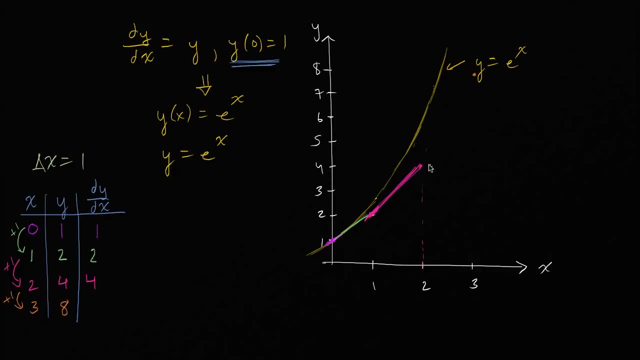 which is right over here, And so for this next stretch, the next stretch is going, is going to look like that And, as you can see, just by doing this we have been able to, we have been able to approximate what the particular solution looks like. 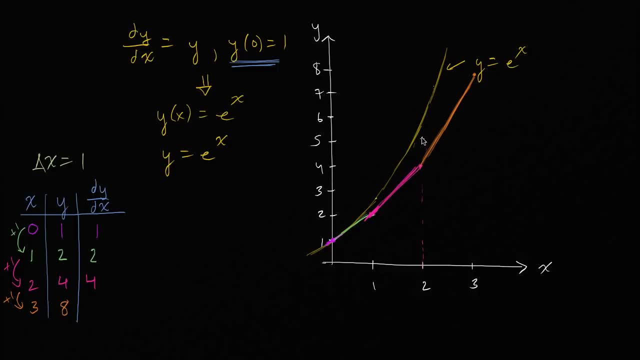 And you might say: hey, Sal, you know that's not so good of an approximation. And my reply to you is: well, yeah, I mean depends on what your goals are, But I did this by hand. I didn't even do this using a computer. 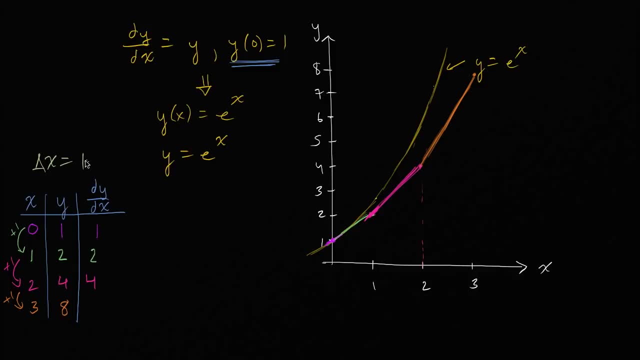 And I, and because I wanted to do it by hand, I took fairly large delta x steps. If I wanted a better approximation, I could have lowered the delta x, And let's do that. So let's take another scenario. So let's do another scenario. 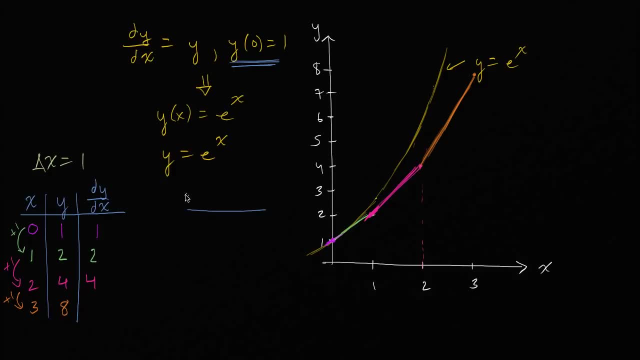 where, instead of delta x equals one, it equals one half. So once again x, y and the derivative of y with respect to x. So now let's say I want to take, so we know, this first point, We're given it. 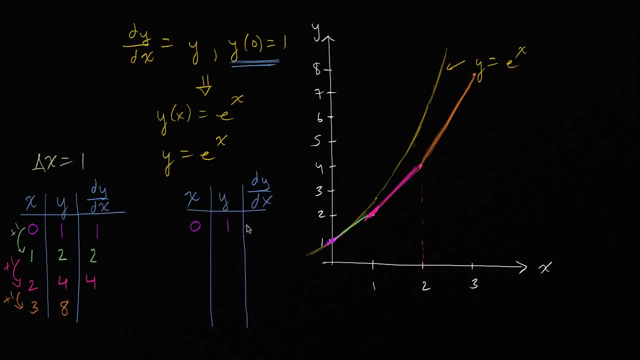 We're given this initial condition: When x is zero, y is one, And so the slope of the tangent line is going to be one, But then if we're incrementing by one half, so then when x is, I'll just write it as 0.5,. 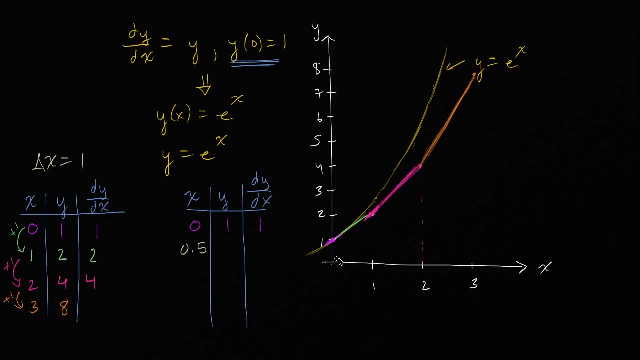 0.5,. what is our new? what is our new y going to be? Well, we're going to assume that our slope from this to this is this slope right over here. So our slope is one. So if we increase x by 0.5,, 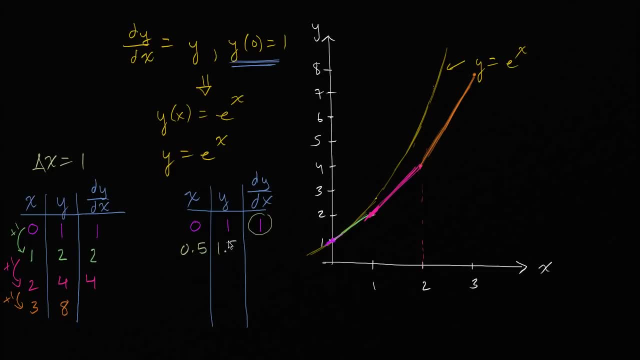 we're going to increase y by 0.5. And we're going to get to 1.5. So we're going to get 0.5, 1.5.. We get to that point right over there. Actually, you're having trouble seeing that. 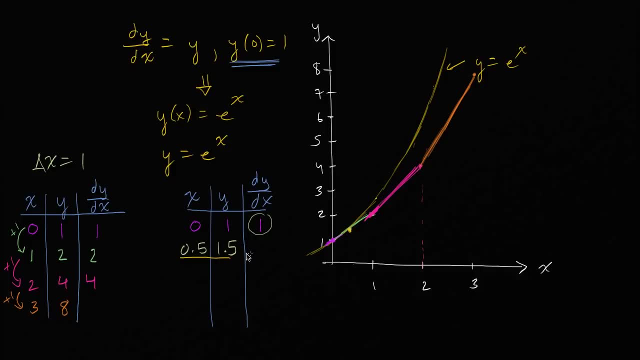 This stuff right over here, is this point right over here, And now our new slope is going to be 1.5,. which is going to look? which is going to look like? which is going to look like actually not quite that steep. 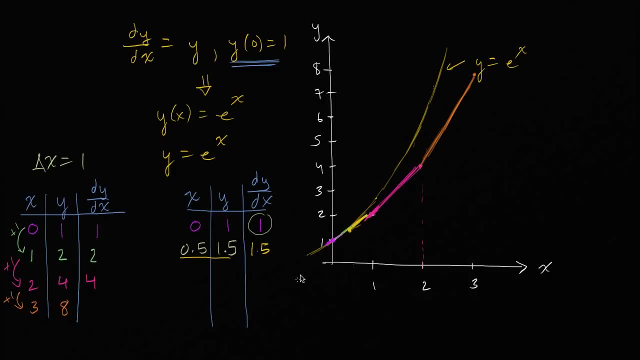 I don't want to overstate how good of an approximation it is and it's starting to get a little bit messy, But it's going to look something like that And what you would see if you kept doing this process. so if your slope is now 1.5,. 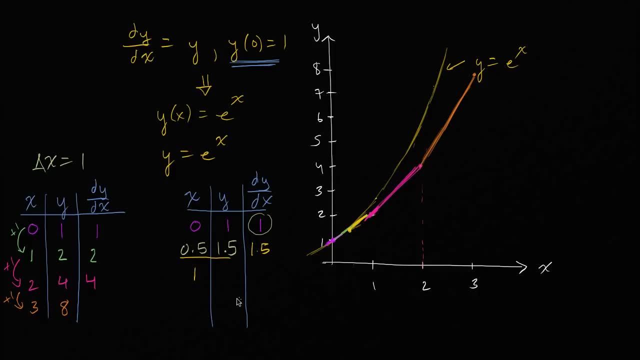 when you increment x by another 0.5, where you get to one. so now, if you increment by, if you increment by 0.5 and your slope is 1.5, your y is going to increment by 0.5.. 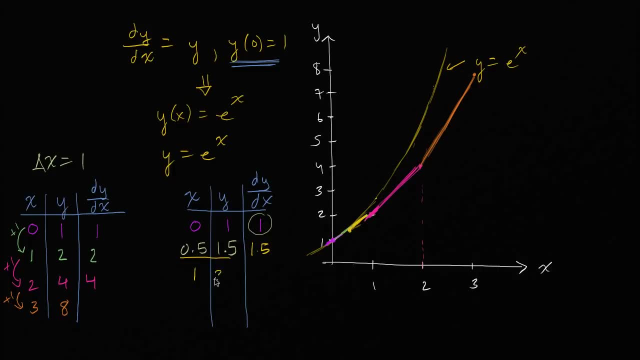 You're going to increment by half of that, by 0.75, and so you're going to get to 2.25.. So now you get to one 2.25, which is this point right over here, And once again. 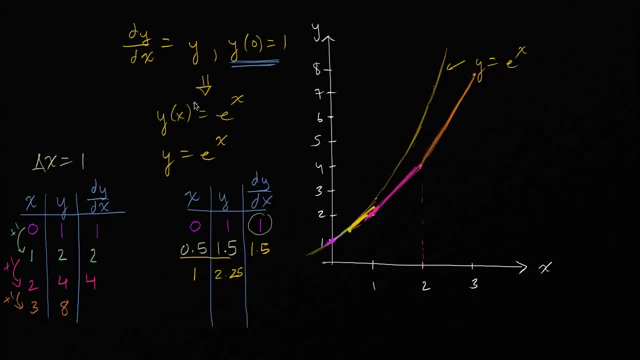 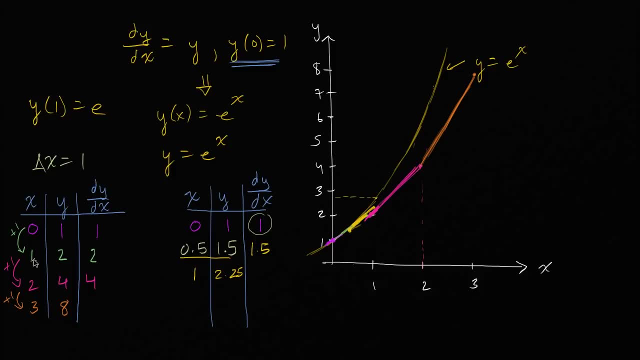 Now, in this one y of y of y of one got us to two. In this one y of one got us to 2.25.. Once again, closer to the actual reality, closer to e, Instead of stepping by 0.5,. 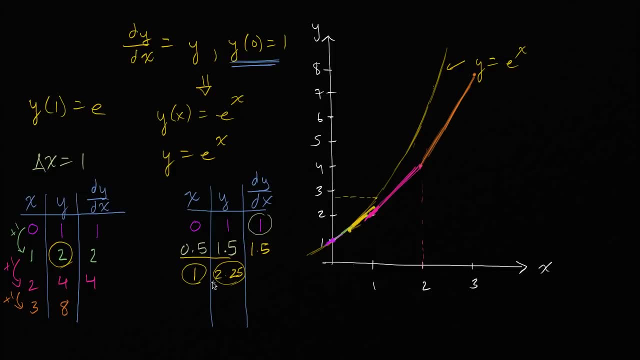 if we stepped by 0.1, we would get even closer. If we stepped by, if we stepped by 0.0001, we would get even closer and closer and closer. So there's a bunch of interesting things here. This is actually how most differential equations 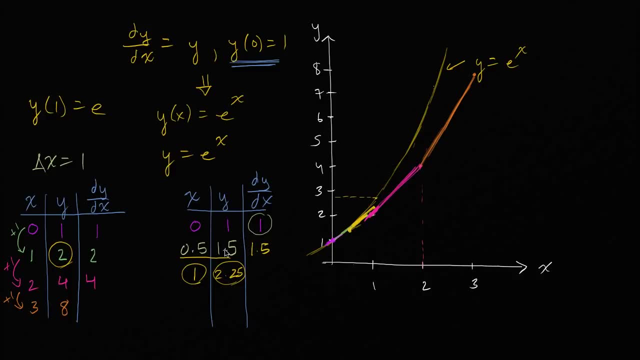 or techniques that are derived from this or that are based on numerical methods similar to this, are how most differential equations get solved And, even if it's not the exact same solution or the same method, the idea that most differential equations are actually solved- or I guess you could say simulated- 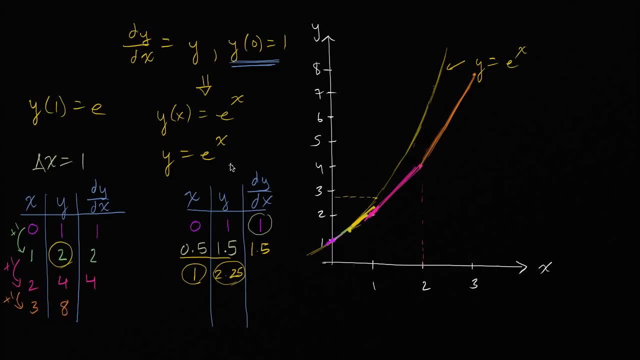 with a numerical method, because most of them actually cannot be solved in analytical form. Now you might be saying, hey, well, what method is this one right over here called? Well, this right over here is called Euler's Euler's method, after the famous Leonard Euler.